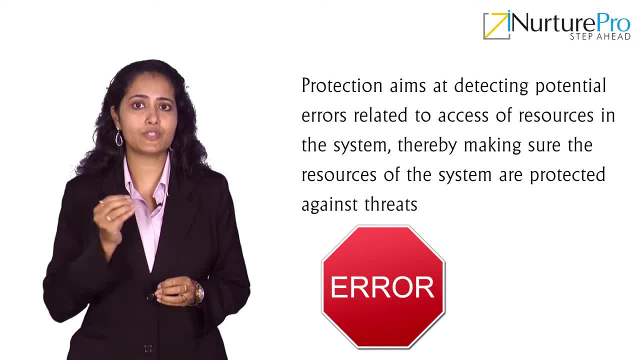 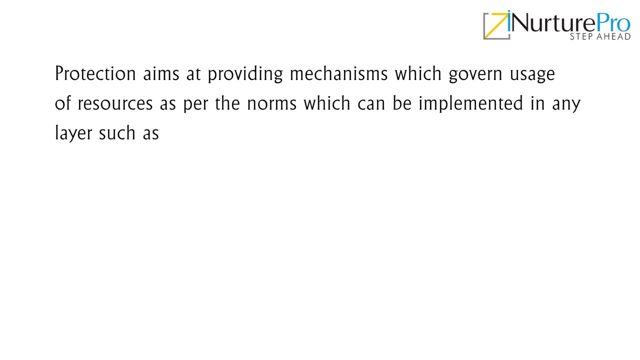 thereby making sure the resources of the system are protected against threats. Protection aims at providing mechanisms which govern usage of resources as per the norms, which can be implemented in any layer, such as design of the OS, individual user management. Next, let us learn the principles of protection. 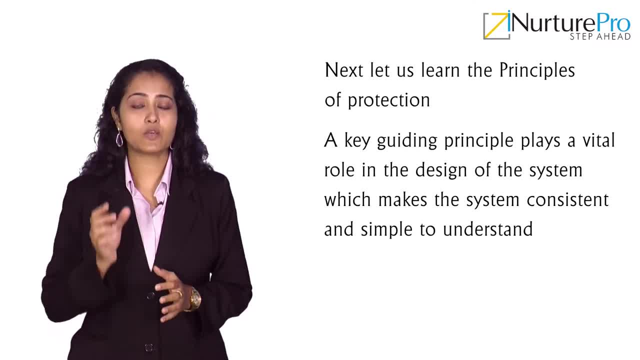 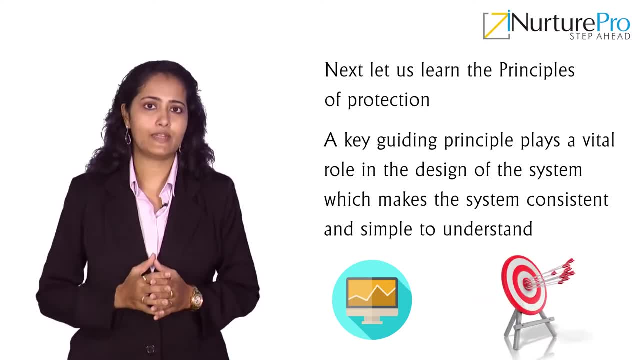 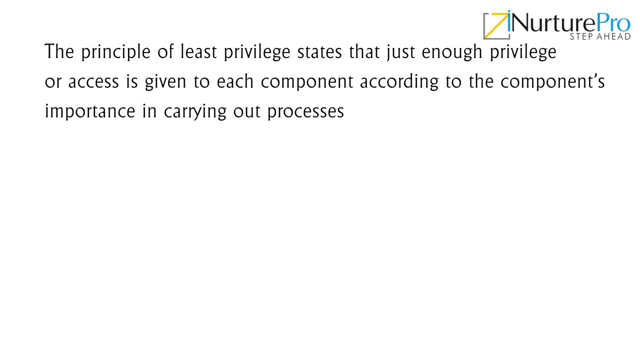 A key guiding principle plays a vital role in the design of the system, which makes the system consistent and simple to understand. One common protection is the principle of least privilege. The principle of least privilege states that just enough privilege or access is given to each component according to the component's importance in carrying out processes. 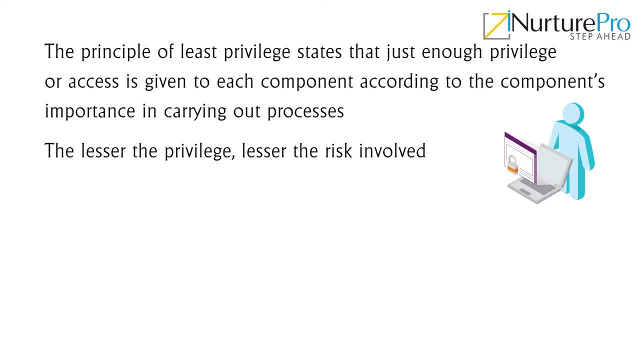 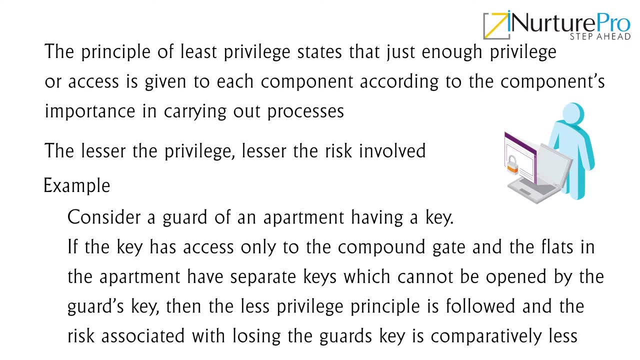 The lesser the privilege, lesser the risk involved. For example, consider a guard of an apartment having a key. If the key has access only to the compound gate and the flats in the apartment have separate keys which cannot be opened by the guard's key, then 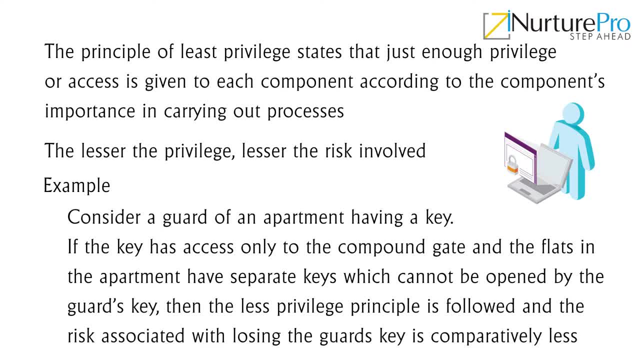 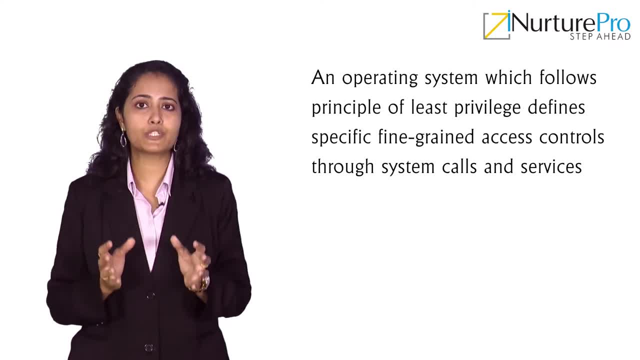 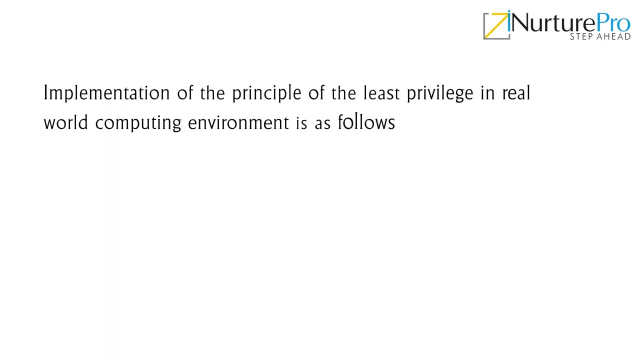 the less privilege principle is followed and the risk associated with loosing the guard key is comparatively less. An operating system which follows principle of least privilege defines specific, fine-grained access controls through system calls and services. This leads to a reliable operating system. Implementation of the principle of least privilege. 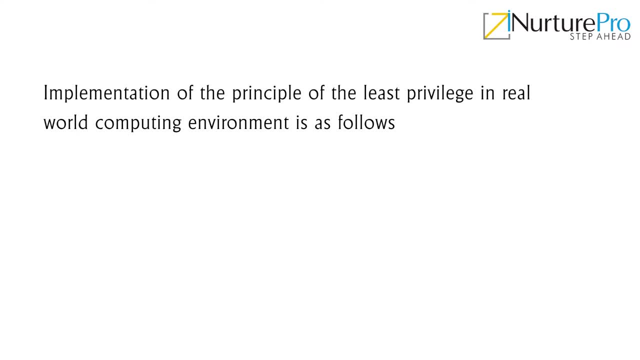 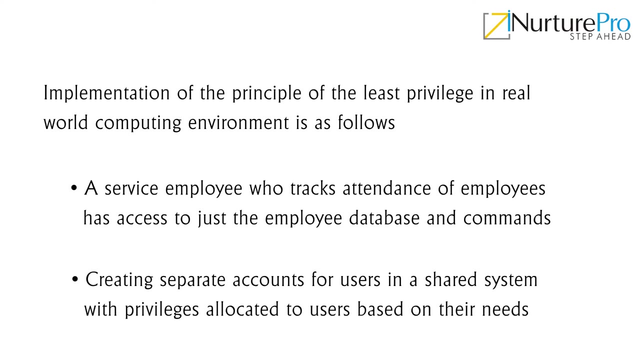 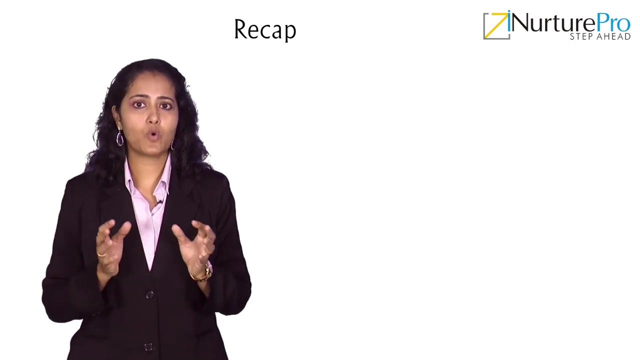 in real world computing environment is as follows: A service employee who tracks attendance of employees has access to just the employee database and commands Creating separate accounts for users in a shared system, with privileges allocated to users based on their need. Let us now have a quick look on what we have learnt so far. 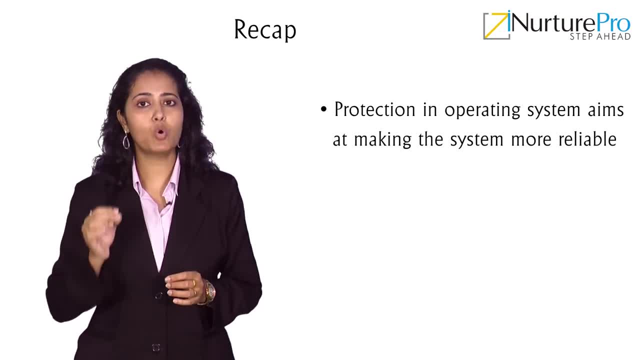 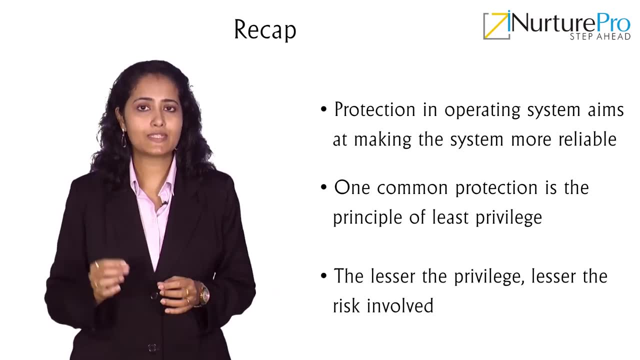 Protection in an operating system aims at making the system more reliable. One common protection is the principle of least privilege: The lesser the privilege, lesser the risk involved. Thank you for watching.